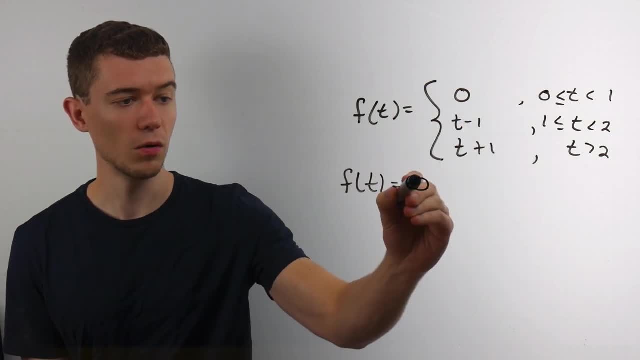 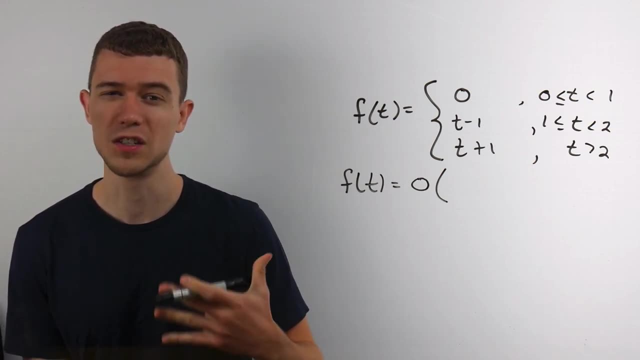 those. So the first one would be zero, and I'll show you the way that I do it. Your teacher might use a different notation for the step function. This is just the notation that I'm going to use. So, the way that I think about this, this u signifying my unit: step function. I think of it. 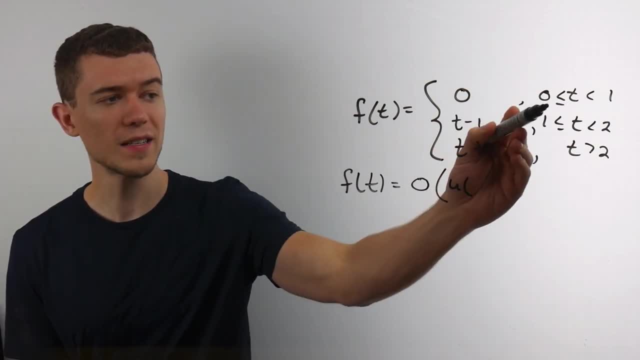 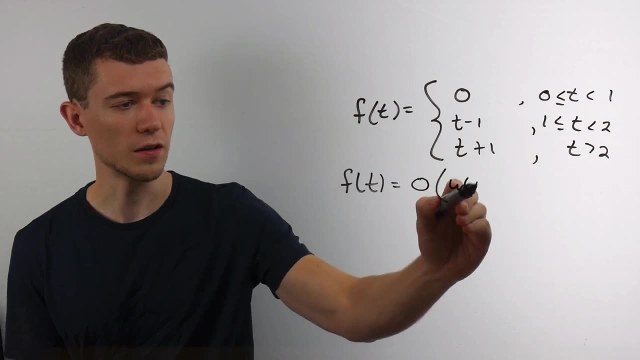 like a light switch, flipping on and flipping off. So where does this first piece, this zero, turn on, flip on. Well, it flips on when t starts at zero. so I would insert a t minus zero. Where does this zero stop? In other words, 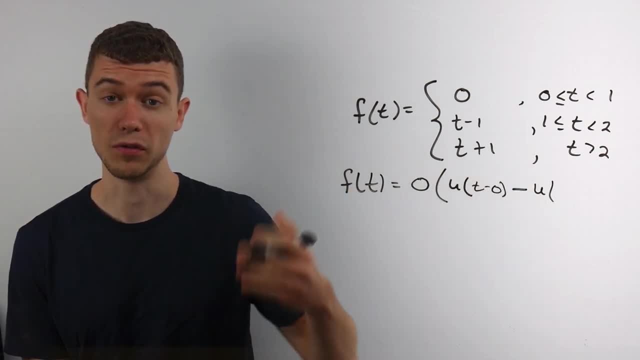 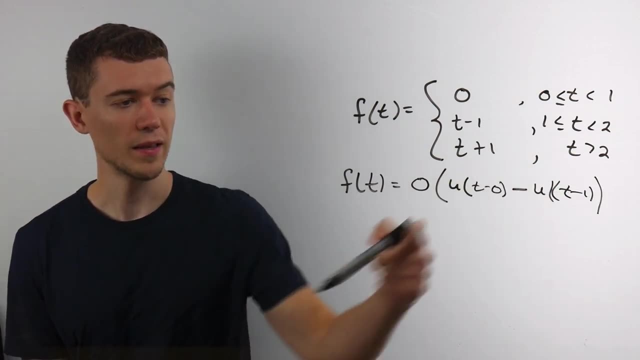 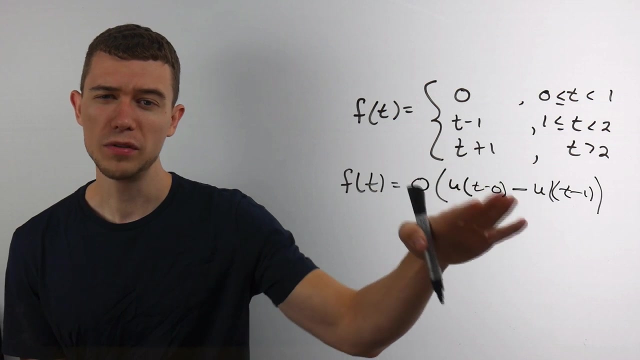 I subtract the unit step function for where it flips off. Well, this first piece flips off a t minus one. So think of the first value, a light switch flipping on. the second value, a light switch flipping off. And again you might use different notation Sometimes you'll just see. 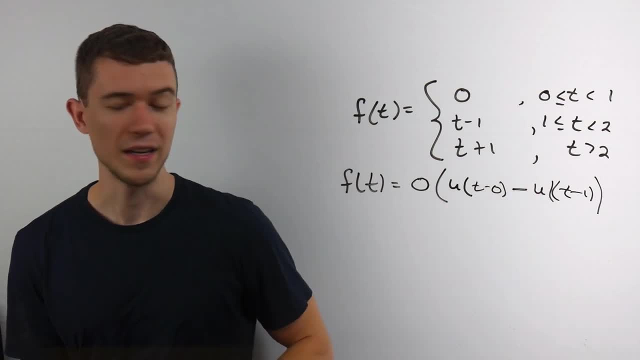 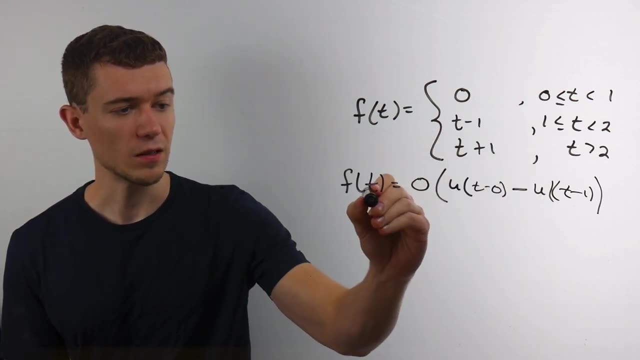 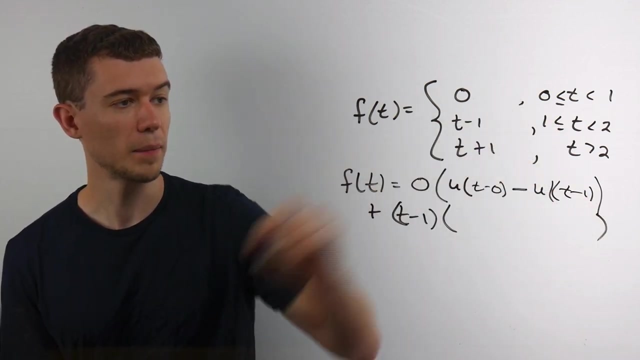 a? u sub zero or a? u sub one here instead of the t minus Both would mean the same thing. How about this second? So I would have plus the second piece, t minus one, and I do the same deal. Where does this second? 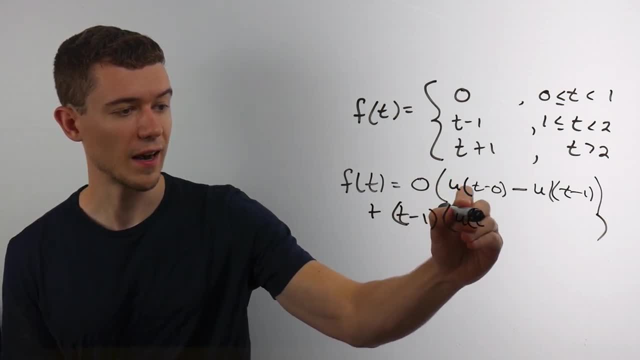 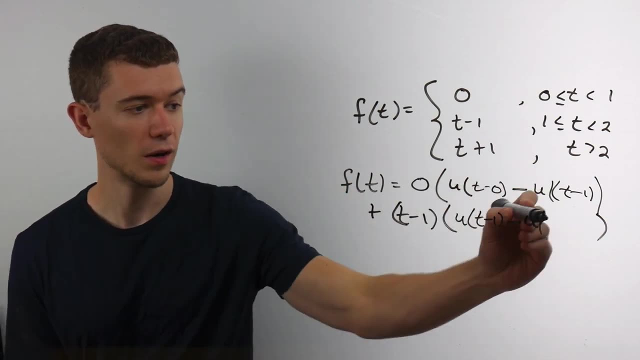 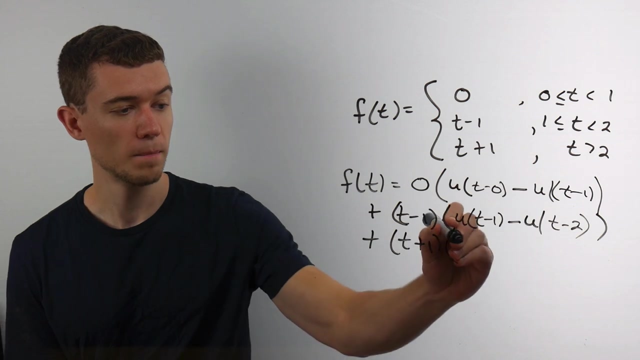 piece activate. Well, it activates at one. so I put a u of t minus one and then I minus to signify the function flipping off at t minus two. Last one, the third piece would be a t plus one. It activates at two. 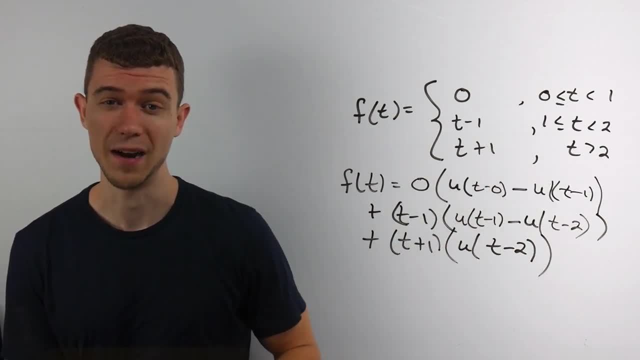 and it goes forever, so it never deactivates after it's turned on. So there we go. We've written this function in terms of its step functions, and you could simplify this a bit. Zero times anything is zero, so this will all just go away, And then I could just distribute the rest, Think. 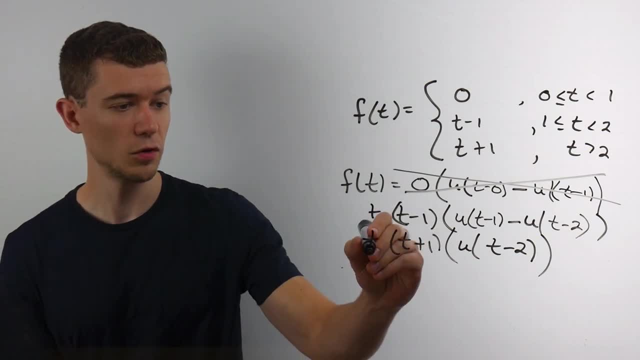 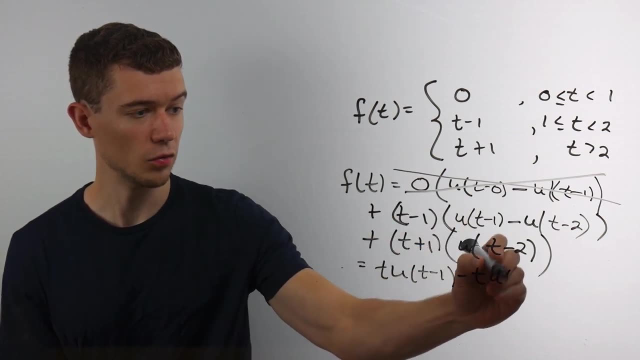 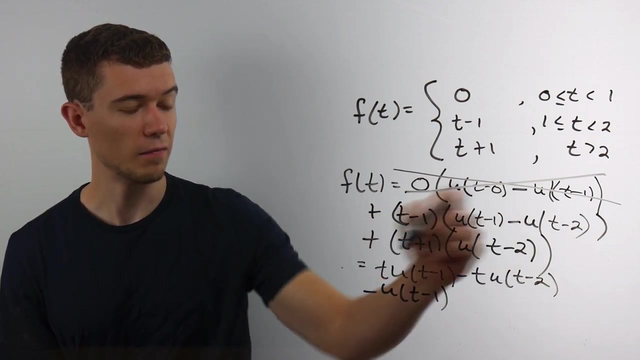 about how the distributive law works. I would have t times u of t minus one, I would have minus t? u of t minus two, I would have minus u of t minus one, And then I would have minus a minus to make a plus? u of t minus two, And then I also have this piece If I distribute. 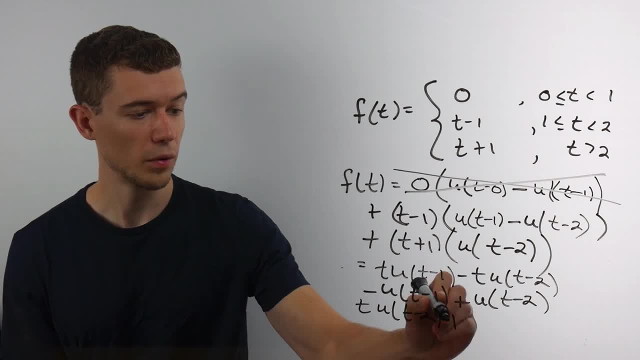 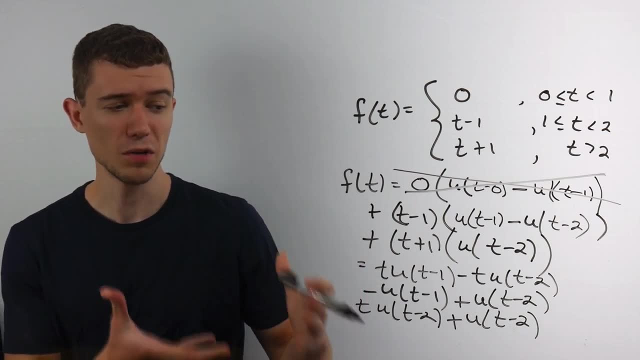 I'd have t times u of t minus two plus one times u of t minus two, So you don't have to do this distributive stuff as much as I did. I did it just because I think it. it makes the Laplace transforms. 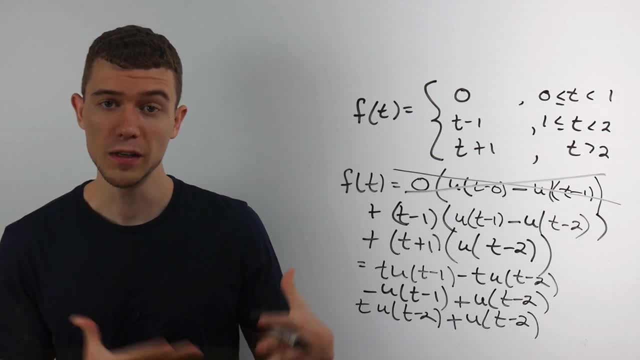 a little bit more straightforward. Your teacher might do it differently. You might be comfortable doing it a different way. This is just how I'm doing it in this example. Well, if you look at this, I have a plus t of u of t minus two. 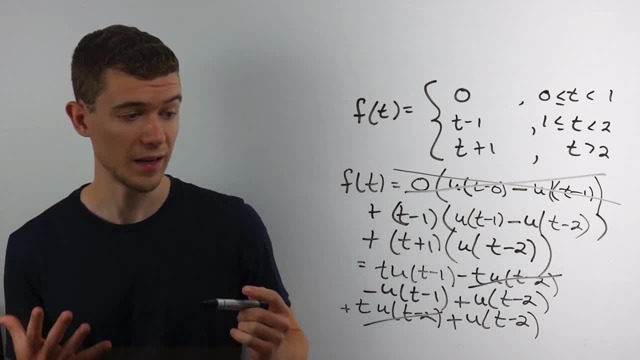 and a minus t of u of t minus two. Those are gonna cancel each other out. And then I'm also having plus two of these, plus two u of t minus twos. So we can rewrite this And we have our simplified function. 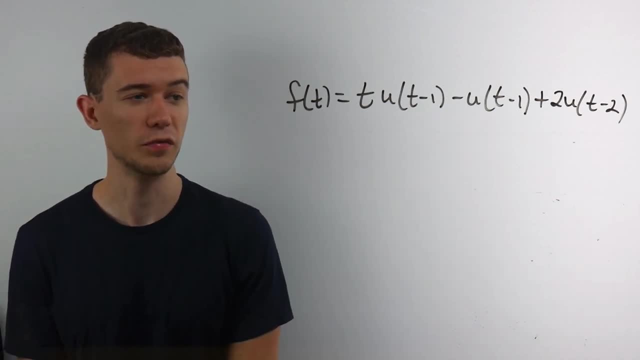 in terms of unit step functions. Again, you could factor out this u of t minus one. I just did it here for the sake of what makes sense to me: doing the Laplace transforms. We're finally ready to do that, to take the Laplace transform of our function. 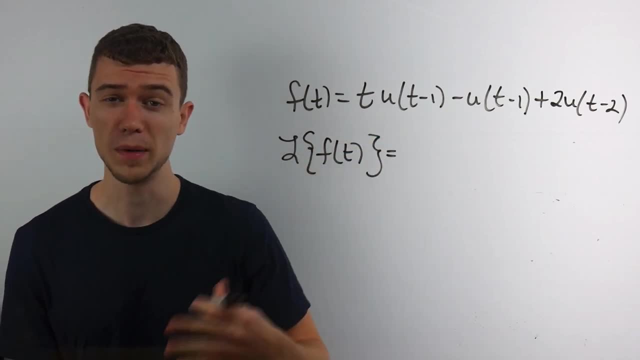 And to do that you have to memorize, or you have to know or be able to look up. how do you take Laplace transforms of functions when they have the step function attached to them? Well, the rule is, if I'm taking the Laplace transform, 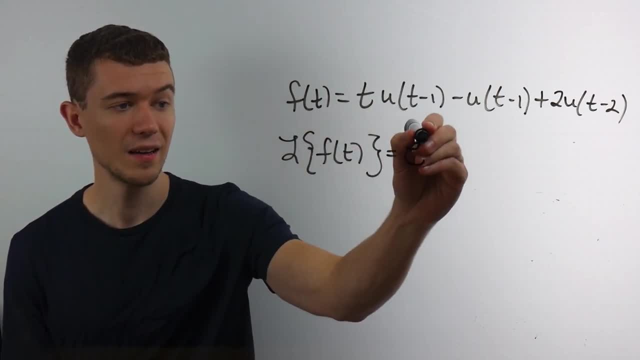 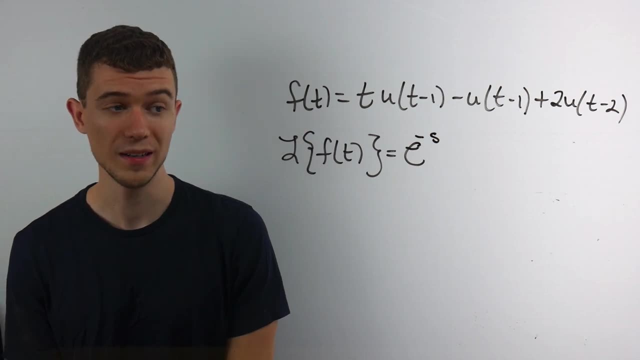 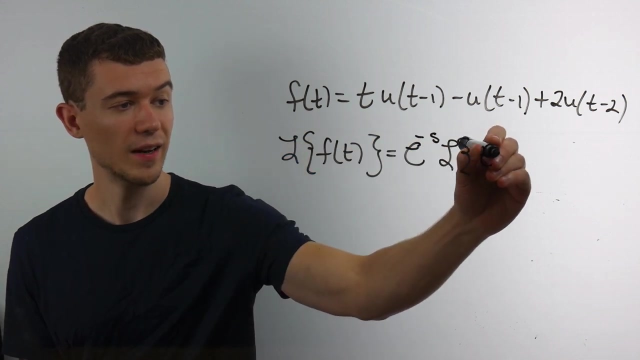 of u, of t minus one that becomes e to the minus, in this case one s. because of this minus one times the Laplace transform of the function, but evaluated at t plus that one, Or in other words, I have to shift. 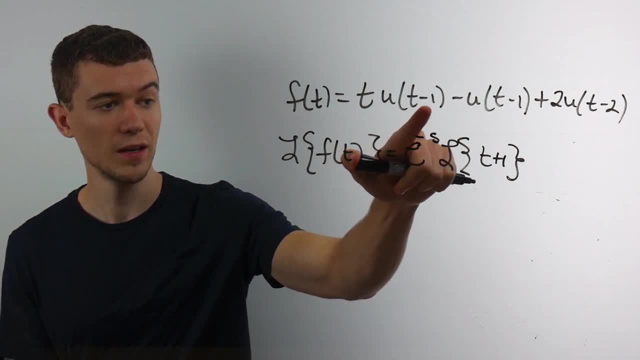 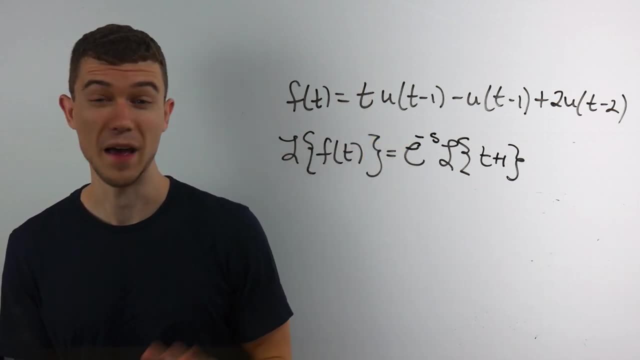 by this amount. So since this one is minus one, this comes out to be an e to the minus s and this function, t, gets shifted by that one in the other direction. Kind of interesting Here, the Laplace transform of minus u, of t, minus one. 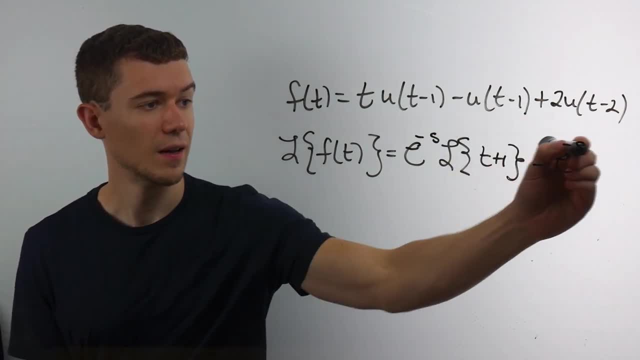 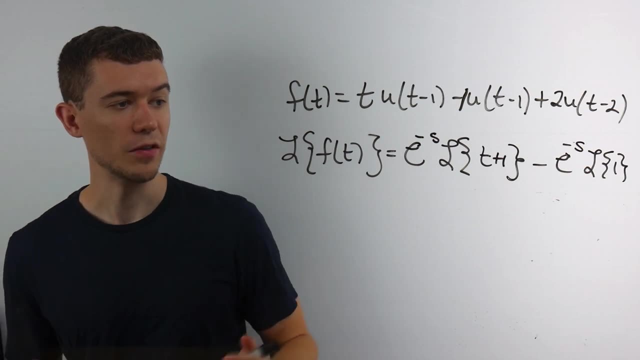 again same deal. we'll have an e to the minus s come out times the Laplace transform of one, There's an invisible one here, And then we have the Laplace transform of one And there's nowhere to shift the one, because there's no t, there's no variable.